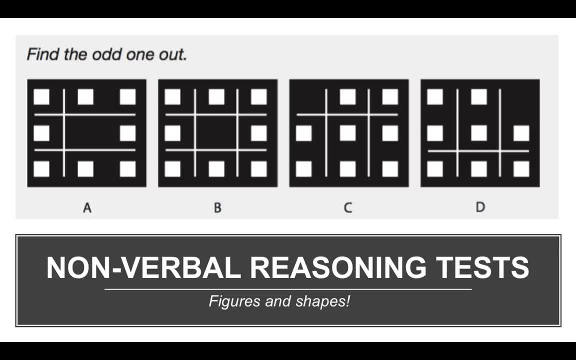 of patterns, of shapes, and then work out what's going on, And these can come in a variety of different questions. I'm going to give you a couple of examples and explain how I've reached the answer, and then I'm going to get you to undertake a quick online mock test. 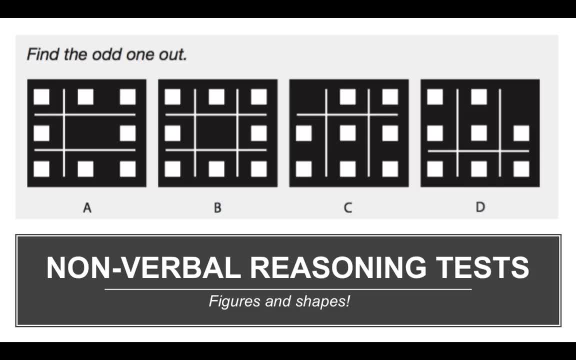 So you can put your answer to each of the questions below the video and I'll mark them for you. As always, I'd really appreciate it if you would give the video a thumbs up And don't forget to subscribe to the channel, because I create these kind of videos virtually. 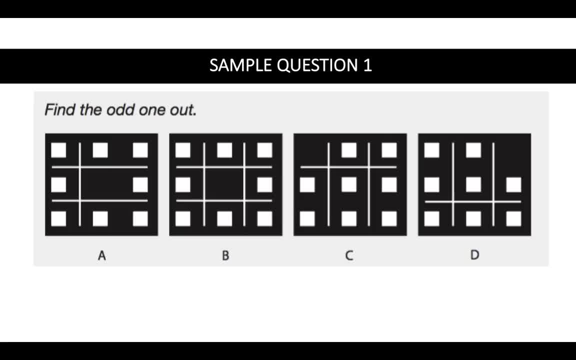 every week. We do quite a few of them and you'll be the first to get notified. So let's take a look at a sample question. So this one here, sample question number one: find the odd one out. So basically, we have to look at all the different patterns from A. 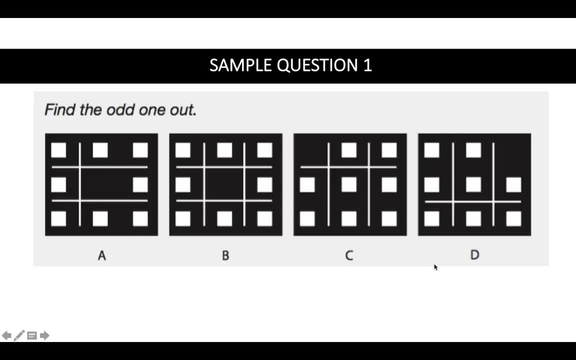 B, C and D and work out which is the odd one out. And a little tip here is that more often than not you're going to get the odd one out And that's because you're going to get the odd one out, But more often than not it is obvious which one is the odd one. 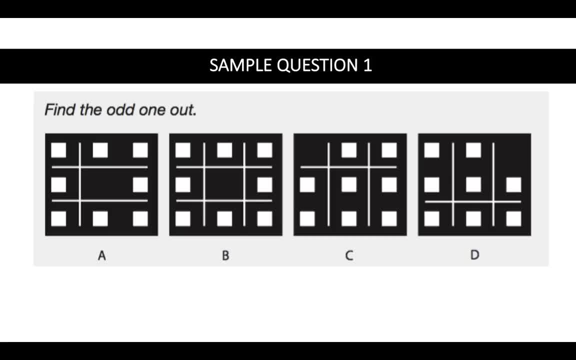 out. You might be looking at this and be looking for different sequences. However, the simple fact is one of the squares contains four lines, whereas the other three contain three, So the best way to work this kind of thing out is to pay attention to everything that's going. 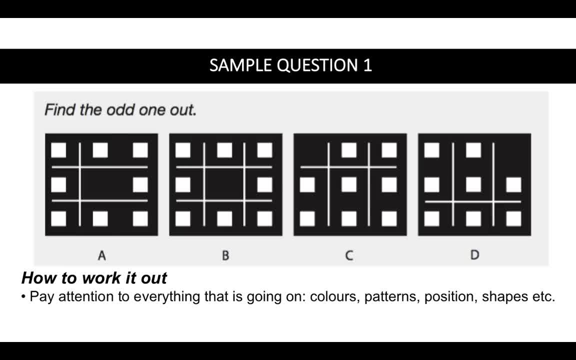 on Colors, patterns, positions, shapes, etc. rotations, And the more you do of these, the better you will become. So at some stage during this video, I'm going to tell you we can get free access to online tests. 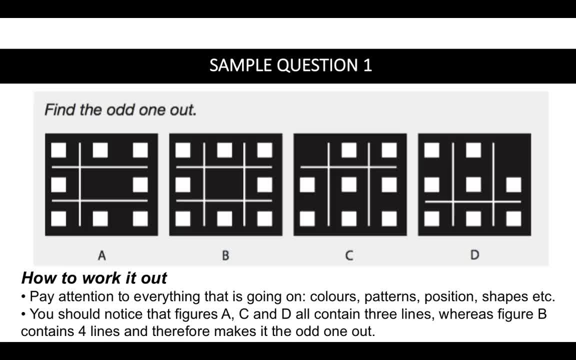 You should notice in this particular question that figures A, C and D all contain three lines, whereas figure B contains four lines and therefore it makes it the odd one out. So it's important because this question might say which one comes next in the sequence. 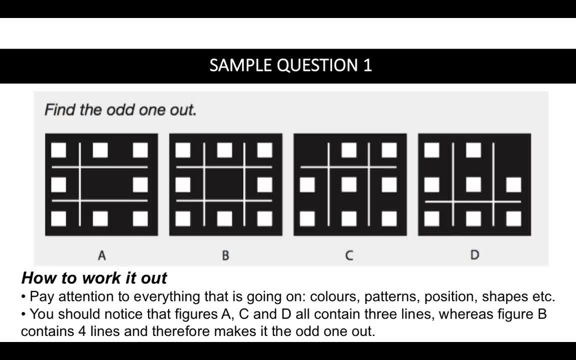 That's a sample kind of nonverbal reasoning question, But this one's just find the odd one out. So the answer there is that B has four lines and it is therefore the odd one out. Don't forget: with this kind of test you're going to be timed, So you have to allocate. 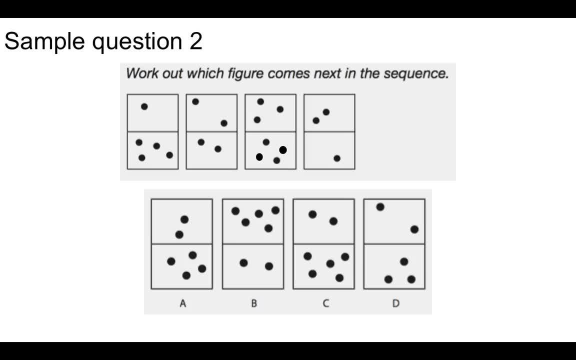 a certain amount of time to each question. Sample question two: work out which figure comes next in the sequence. So we've got these sort of like domino symbols here at the top. You've got one, two, three, four and we need 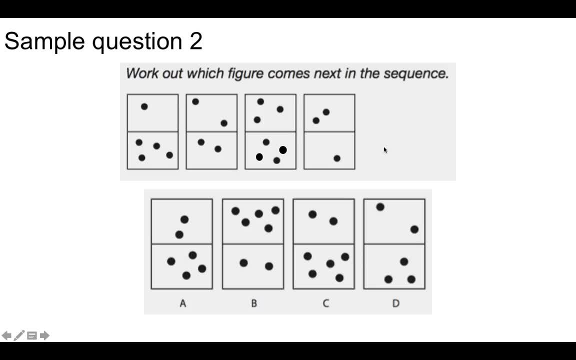 to work out from the sequence below A, B, C and D, which one comes next. So what you have to do is to look at the pattern, And the first one would be to look across the top to see if there's a pattern. So we've got one, two, three, two. That's not really. 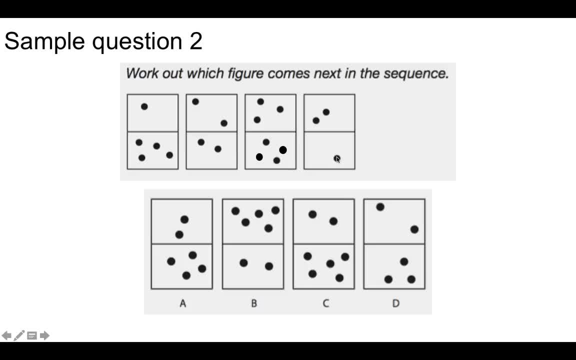 a pattern. We've got there four two, four one. That's not really a pattern, So what I'll do next is try diagonally At the top left: one, two, three, one. That could be one, two, three, one, And I would. 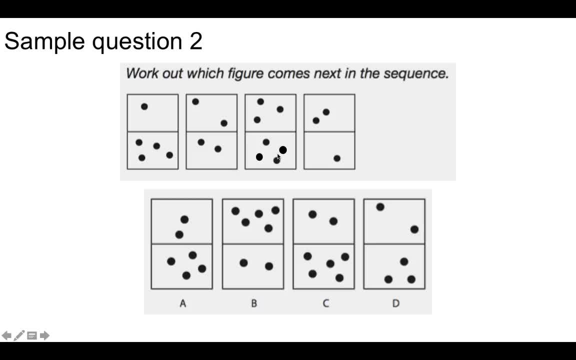 expect one up there to be two. We've got here four, two, four, two. So I'd anticipate at the bottom there would be a four. So therefore I'm looking for a two at the top and a four at the bottom. You can see there that I've got one, So that one A would be my answer. 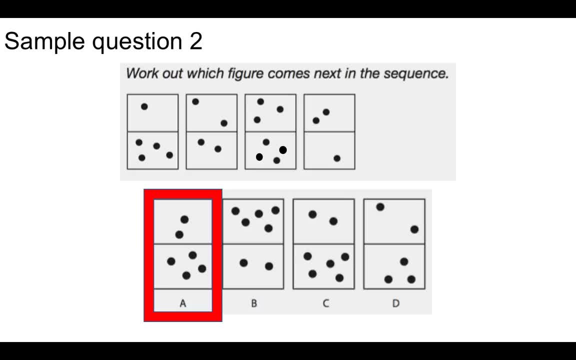 to that question. So it's just about a process of elimination, starting at the top and then going diagonally to see if there is an option. Just a quick point: You might find that in some questions you'd have E as an option. 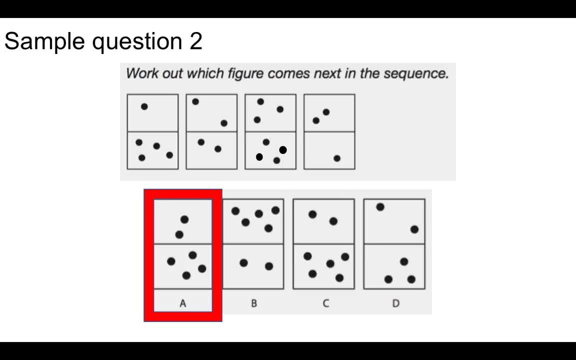 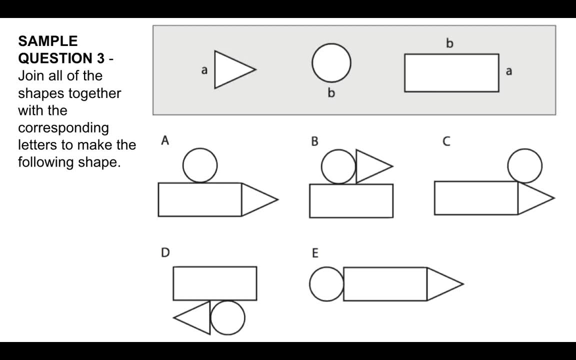 which would be none of these. That's slightly harder to work out because if you can't find the right answer in any of them then you'd have to take the risk and say it's none of these. Sample. question three: This is a different kind of non-verbal reasoning test. Join all. 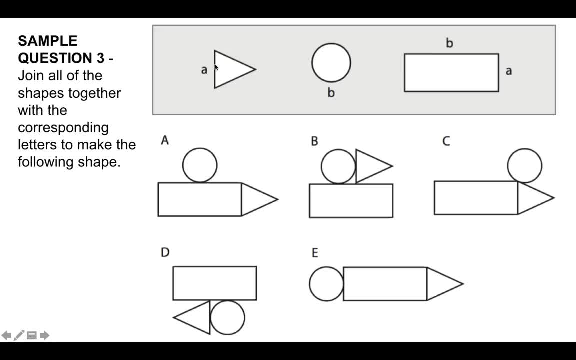 of the shapes together across the top in the gray shaded box with the corresponding letters, to make any of the following shapes: We've got A, B, C, D or E. So if you just look at the top here, what I'm going to do is I'm going to drag that triangle across and fit. 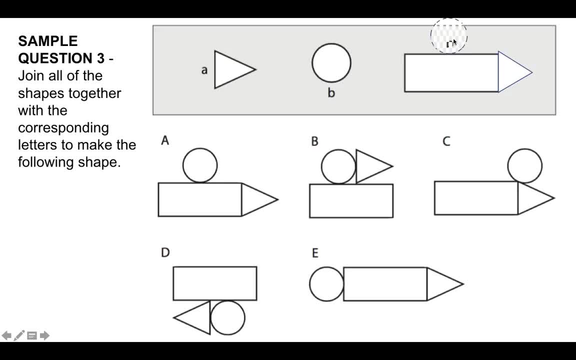 it on there like so, And I'm going to take the circle and position it with the corresponding letter. So I'm looking for a shape that looks like that, And I've got one there which is A, So that's the correct answer. The more you work these out is start to do these in. 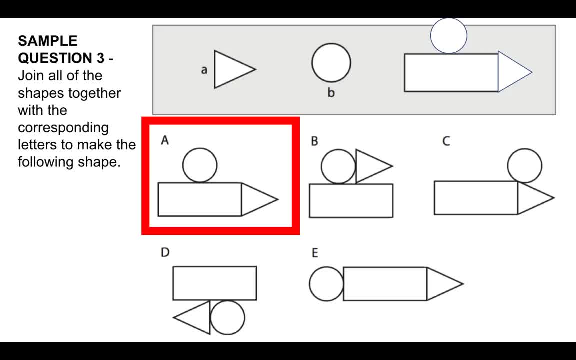 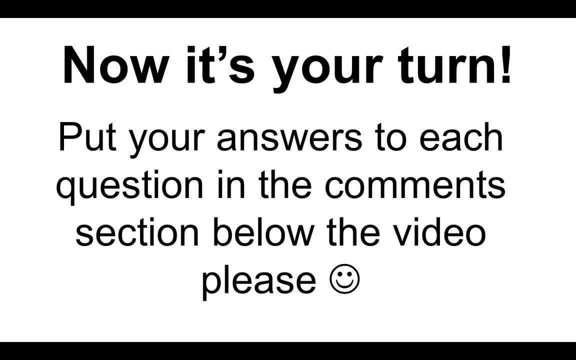 your head, They become relatively easy. Like I say, the more practice you do, the better you become at it. Okay, So now it's your turn. I'm going to give you seven sample questions. Excuse me, Seven sample questions. Put your answers to each question in the comments section below. 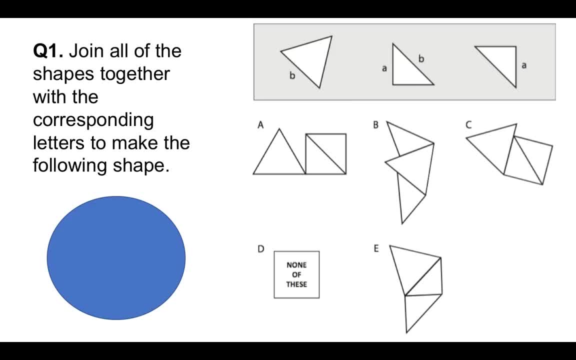 the video, please, and I'll mark it for you Now. I have given you a time limit to each one, which is 15 seconds. If you find it's not enough time, just simply pause the video and work out a question. I'd. 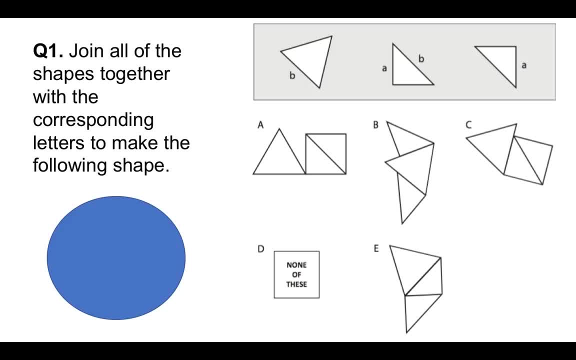 like you to get them all correct and work all through them. So question number one: Join all of the shapes together. We've just done one of these across the top of the corresponding letters to make the following shape: You've got 12 seconds And don't forget, there is 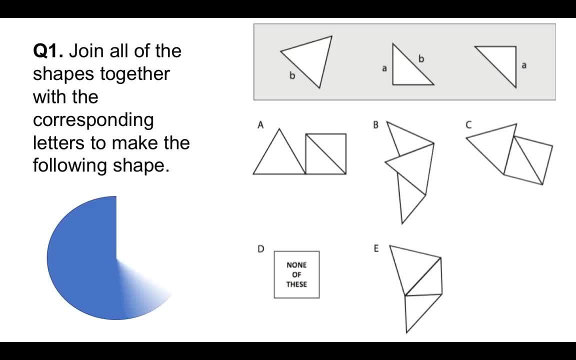 one there which is none of these. So just join up all of the shapes of the corresponding letters and let me know which is your answer in the comments section to question one. Okay, Question number two, Same kind of question. Let's try this again: Join all of the shapes. 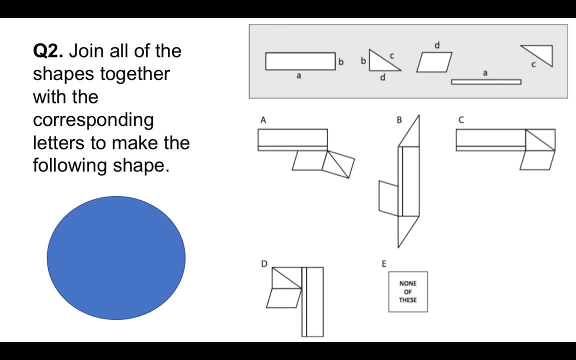 together with the corresponding letters to make the following shape: Again, we have an option: A, B, C and D, E is none of these. So again, you've got 15 seconds. Join them all up and let me know which one you come up with. 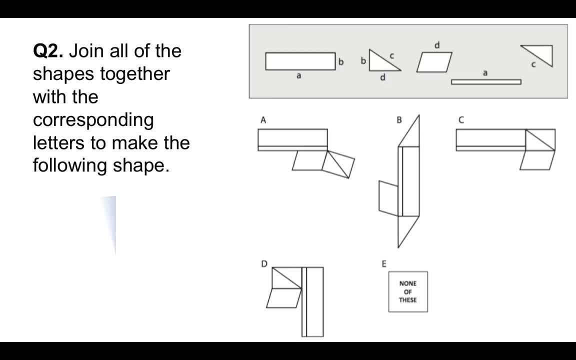 So, like I say, the more you do of these, the better you will become, And I'm going to give you a sample test soon, free of charge, where you can try more of these. Hope you did well with that one. Question number three: 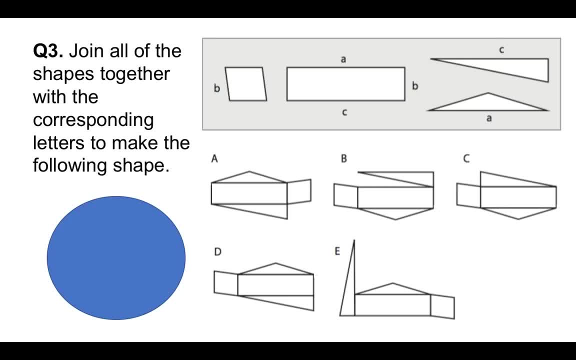 Another one. Join all of the shapes together across the top of the corresponding letters to make any of the following shapes: You'll see there that you haven't got a none of these options, So it is one of them which is right there And you might have to rotate the finished. 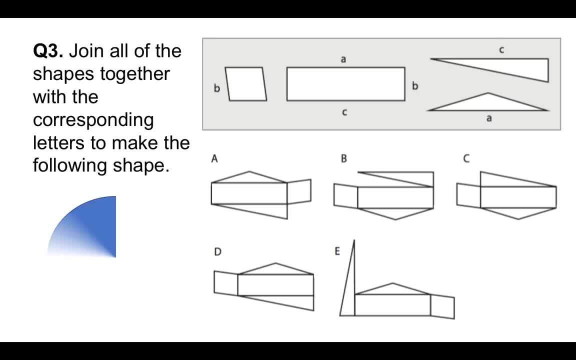 shape in your mind to get the correct answer. But, like I say, we want to get you to the point where you're doing these in your head without having to write them down. But if there's not enough time, don't forget to pause the video. Question four: a different type. 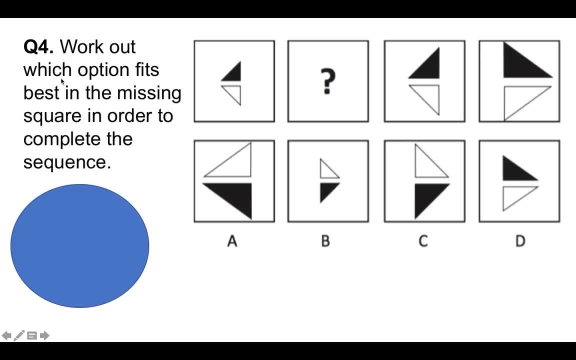 of one now. So it says here which…. Okay, Which option fits best in the missing square? That's the one there with the question mark in order to complete the sequence. So you've got these two here across the top. Which one? 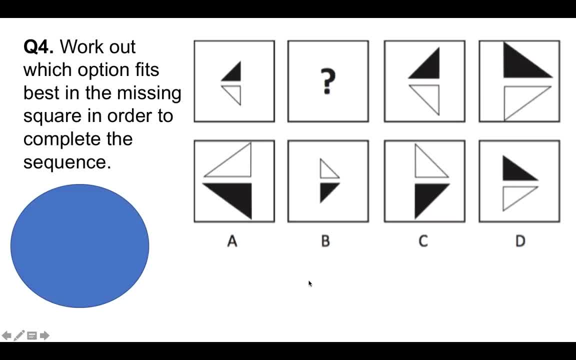 is it A, B, C or D? across the bottom that goes there. So don't forget what I told you before. You've got 15 seconds. Work out. if there's any patterns- And there's a pattern straight away for me, which you know- it's black across the top. Okay, Fantastic So. 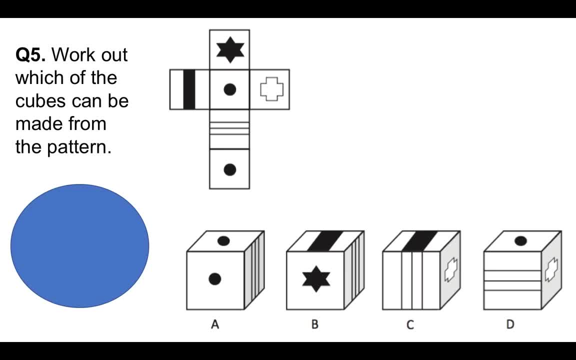 let's go back to question number five. Question number five: work out which of the cubes from the bottom can be made from this pattern. So you're gonna have to make this pattern in your mind and work out which one it is from- A, B, C or D. You've got 15 seconds.